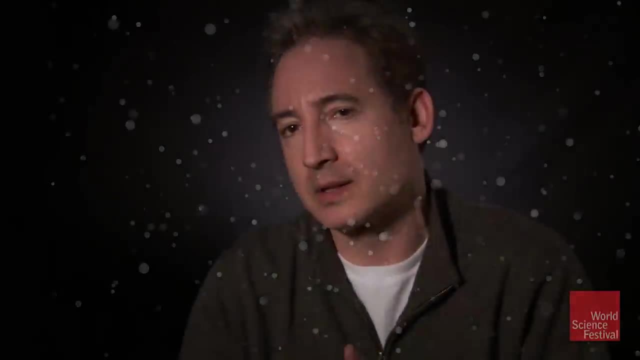 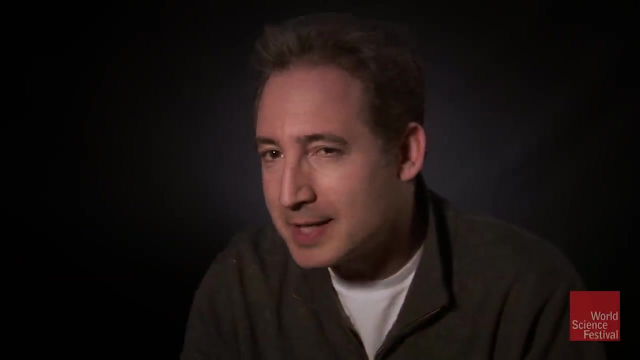 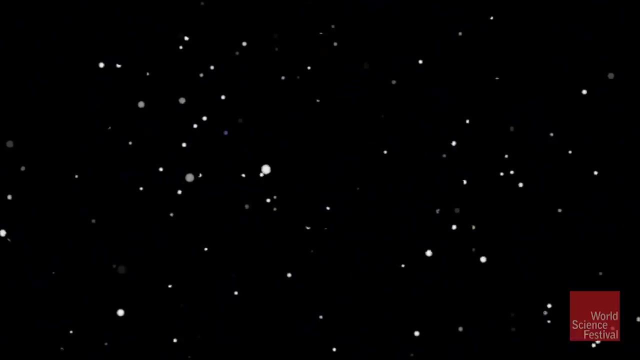 it gets crushed out of existence. Every object in some sense contains information, because it contains a very specific arrangement of particles. So where is the information that describes the arrangement of those particles? Where does it go? Hawking's description of this process was that the energy remains but the information. 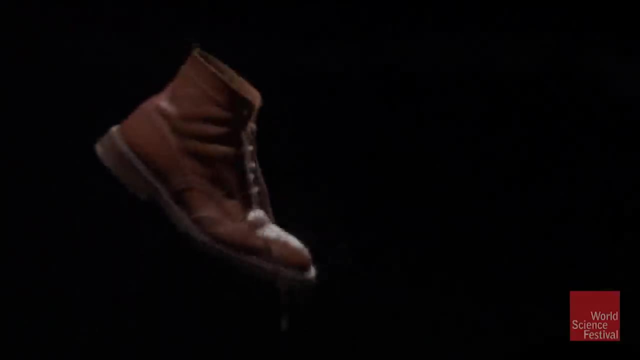 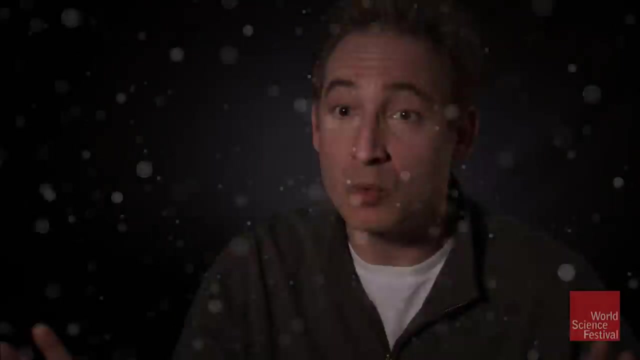 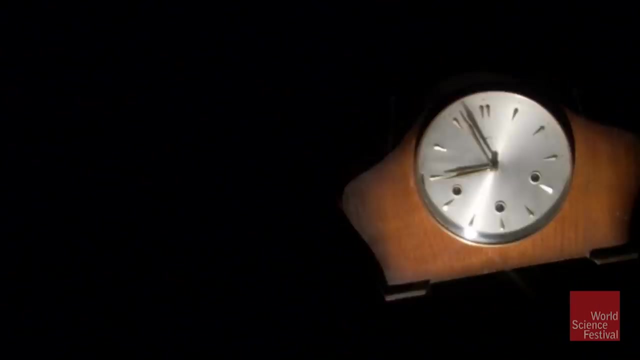 disappears. For many years, for decades, people wondered: is Hawking right? Is the information obliterated and disappears from the universe, or is it still there and perhaps can be in some way retrieved? The destruction of information was counterintuitive and it didn't match the rest of the things. 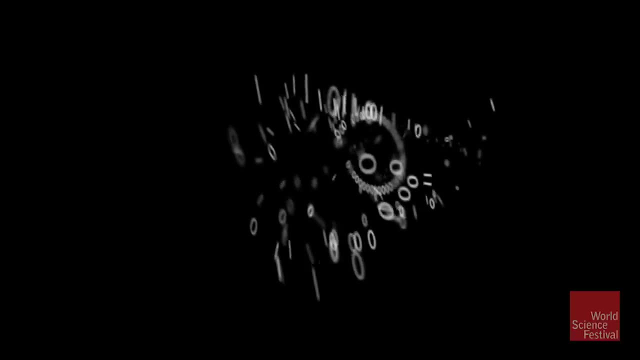 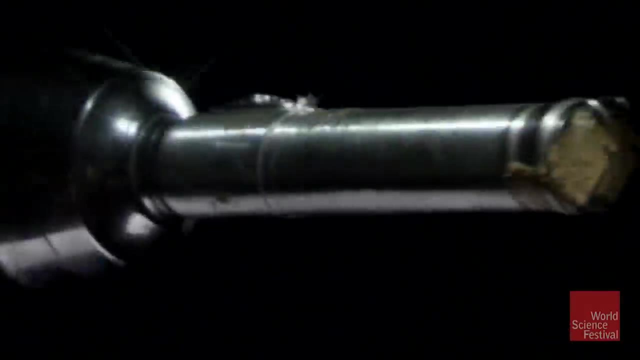 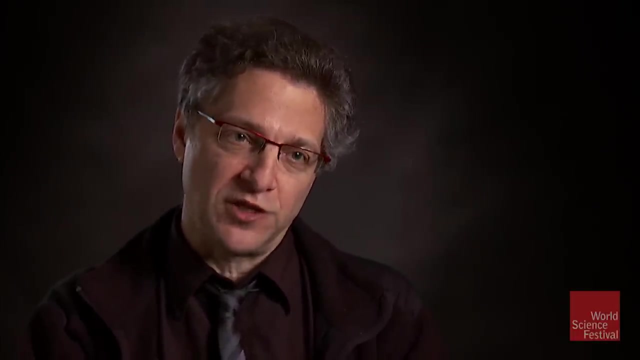 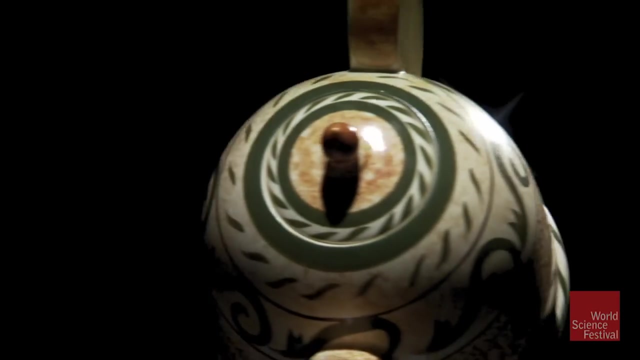 we knew In all parts of physics we had a situation where information doesn't get destroyed, so it was a bit puzzling. This debate furiously went back and forth up through the 80s and into the 90s when people finally began to articulate this new principle, this holographic principle, And what it said. 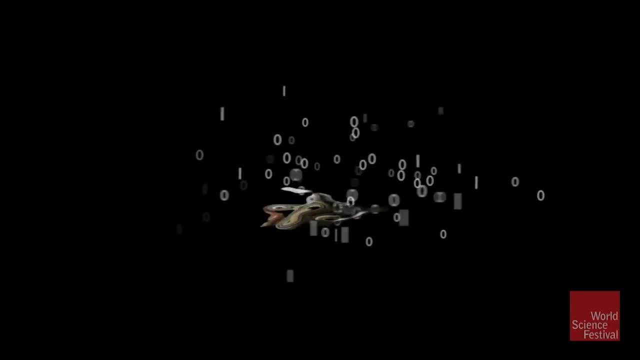 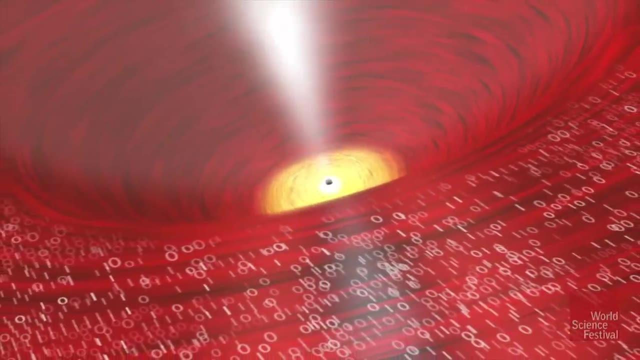 is that all the things that we know about the universe, the universe itself, the universe itself, all the things that we're following inside a black hole were somehow captured in a preserved image at the horizon itself. So if the information is not lost on the surface, the information is not lost inside, because 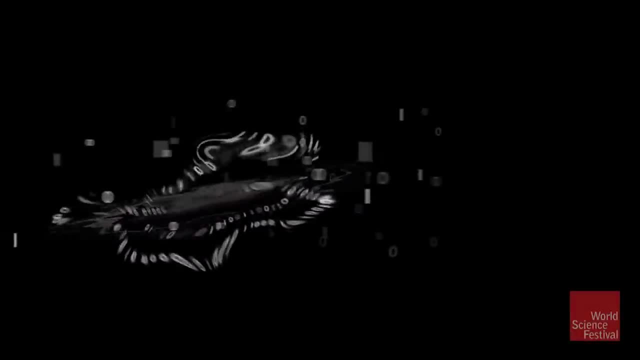 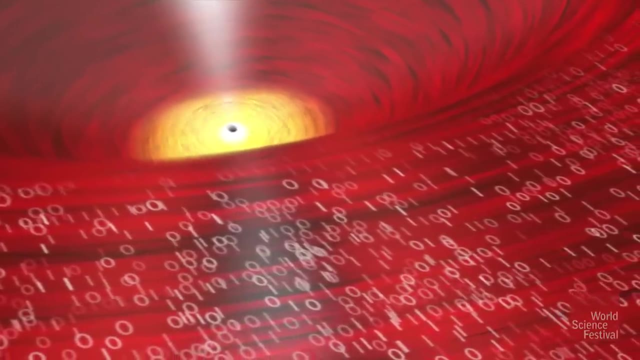 they are equivalent. All of the information about those objects, what they were like in their three-dimensional existence, was preserved or encoded on the surface of the black hole, And that's a little bit like a hologram. Well, that suggests that maybe that idea of the black hole, the black hole itself is. 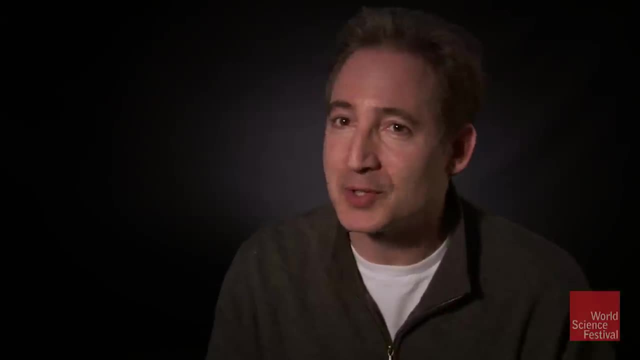 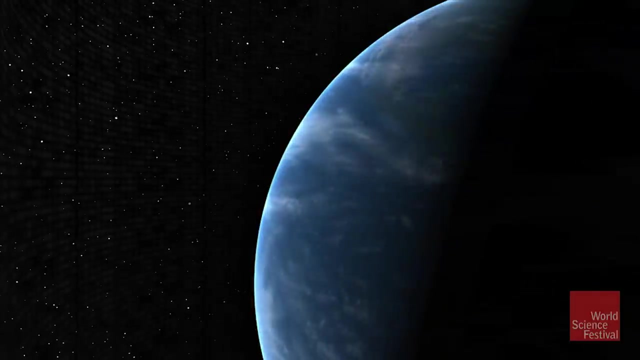 not lost. That idea may apply more broadly to the universe as a whole. Maybe the three-dimensional objects us everything in the world around us. maybe all of the information in these objects is carried, is smeared around a distant two-dimensional surface that surrounds us and we're just. 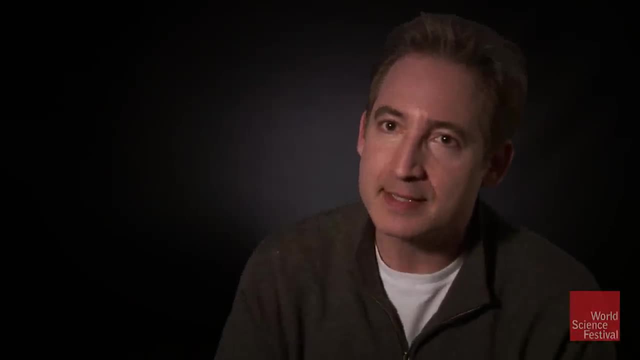 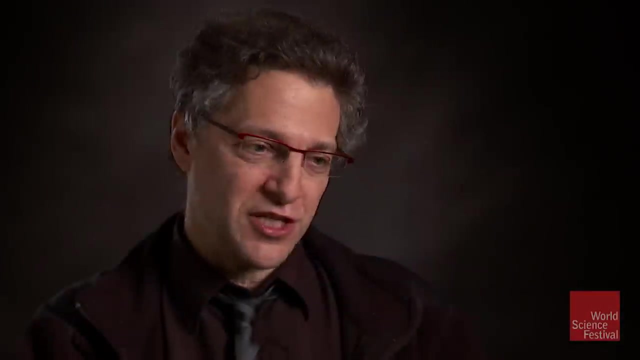 in some sense a holographic projection of that distant data. The holographic principle tells us something quite astonishing. It says that our ideas of volume, of the universe, of the universe itself, are not lost. They're not lost, They're not lost. 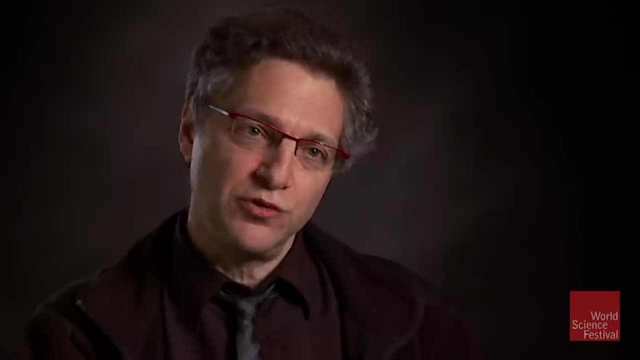 The volume of the real world, in a sense might be a kind of illusion.